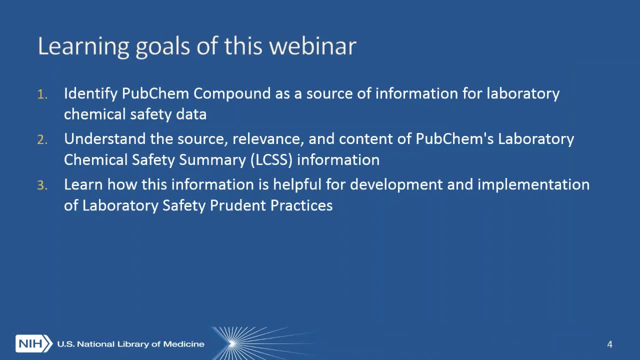 you can check back, you might find something. the next. So the hope is that from this webinar, you'll be able to understand three primary things. That PubChem compound is a source of information for your laboratory chemical safety data And the hope here is that you can understand the LCSS, the PubChem's Laboratory Chemical. 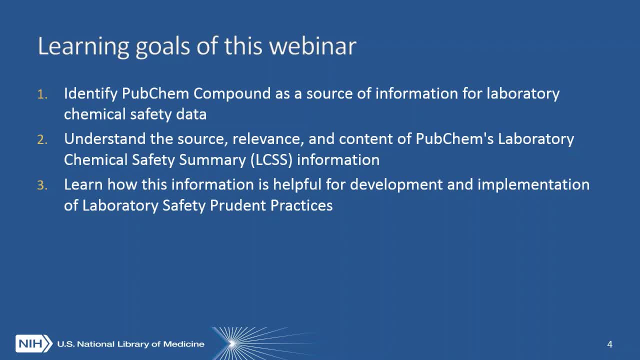 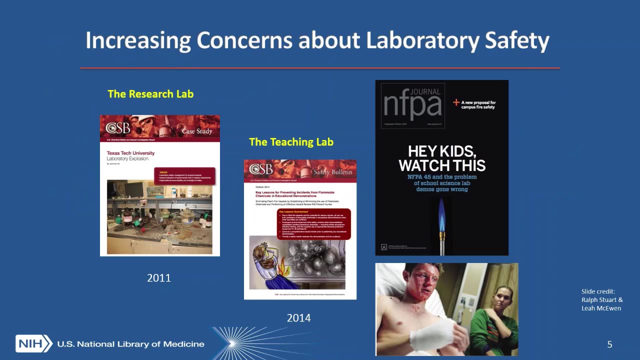 Safety Summary: The source and content where you can access information, but also how you can use and access relative to laboratory safety-producing practices. There's quite a number of reasons for this webinar to be important for many people. For one, there are three hazmat responses to laboratories every week. Academic research laboratories. 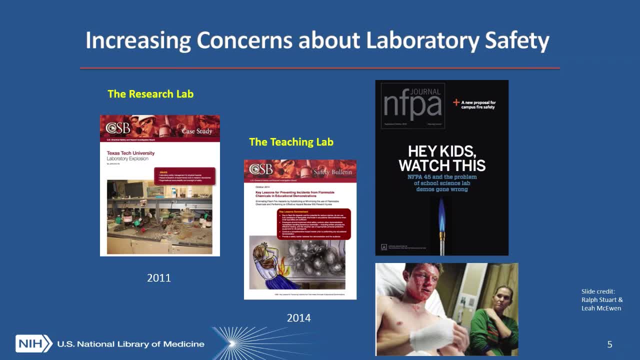 account for about of all HAZMAT responses to laboratories in the US, and teaching labs account for about 10%. Education is the third highest HAZMAT response sector. Since 2010,, the Chemical Safety Board has produced two major reports on chemical safety. 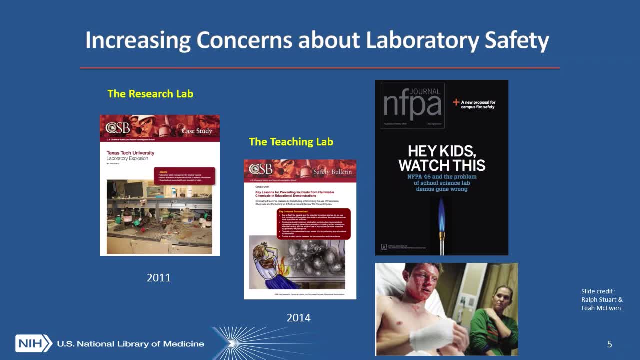 incidents in research and teaching laboratory settings. These are based on a classroom methanol fire in 2006 and a series of research lab events from 2008 to 2011.. There have been an ongoing series of laboratory HAZMAT events since then and it has accumulated. 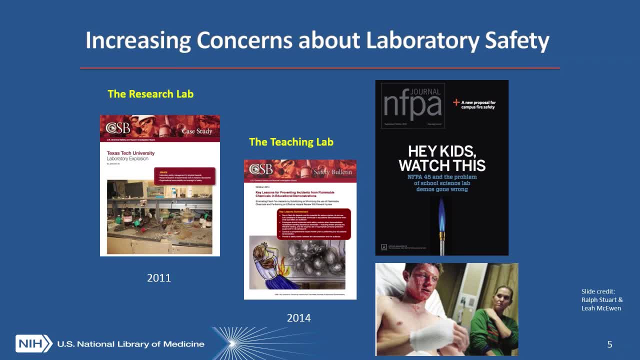 a history of chemical accidents which have really called into question the traditional laboratory health and safety paradigm of don't make mistakes and we won't have accidents into question and led more to concern about the safety culture of laboratories. This has been specifically addressed in reports by the ACS and National Research Council. 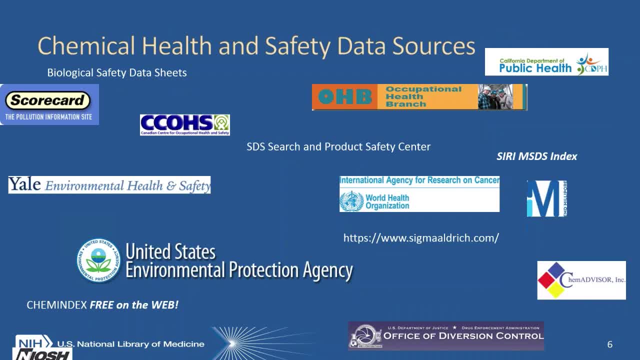 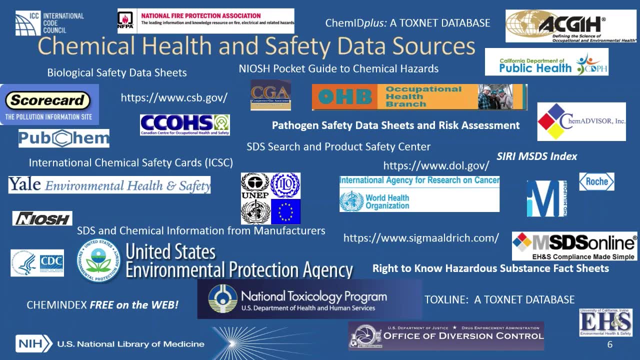 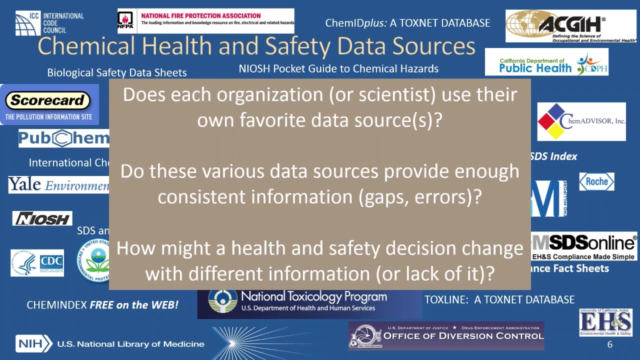 So chemical, health and safety data sources are really blessed in many ways of having so many different data sources available. This, however, presents an issue in that there can be gaps or errors in information. If all the information was available, will decisions made by chemists change? 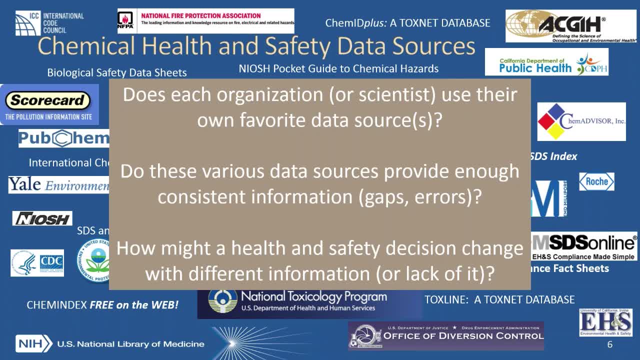 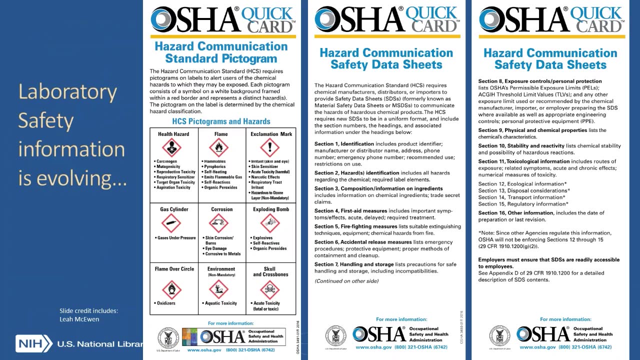 Every scientist you can think of. they may not be aware of the various sources of information I just presented here- Just a small fraction of those that are available. Couple into this the fact that laboratory chemical safety information is evolving. There's been a recent transition from material data to safety sheets, the so-called MSDS. 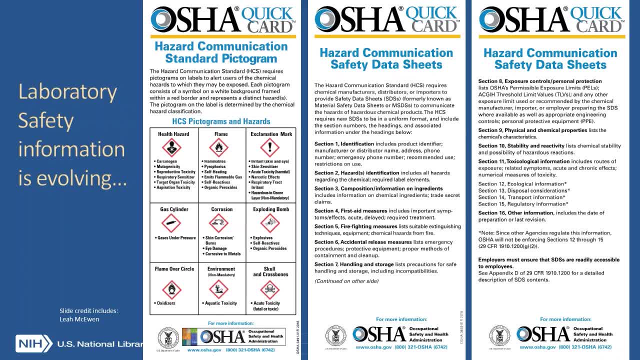 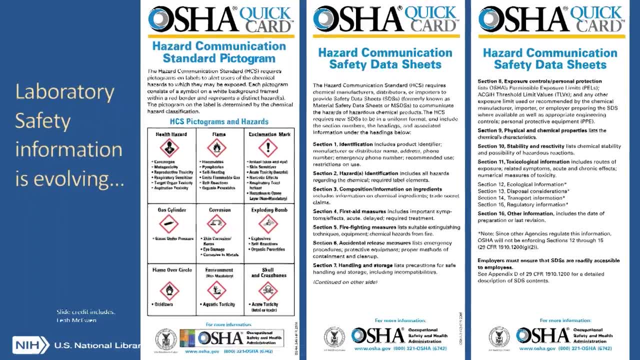 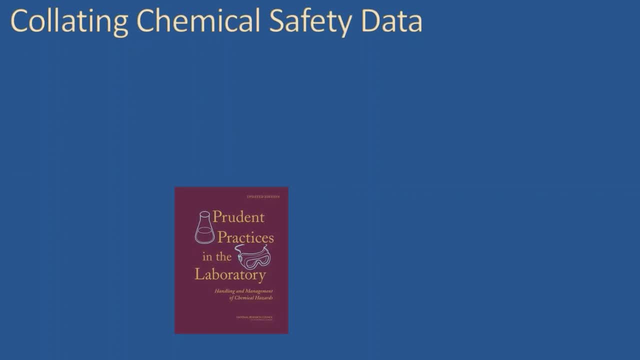 to the global harmonization system, GHS safety data sheets, otherwise known as SDS, And this was really a major step forward, in part because it provided a standardization of the information content that would be available. Okay, So this has been further evolving through the National Research Council, NRC's putting. 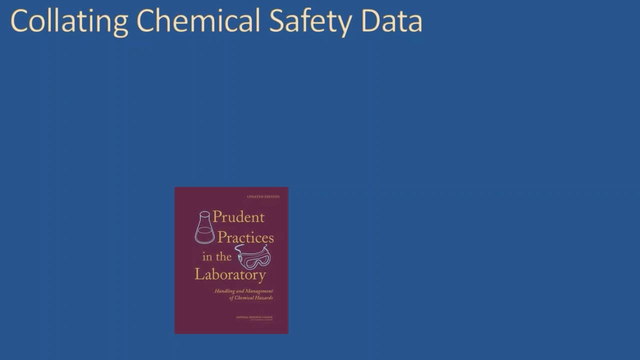 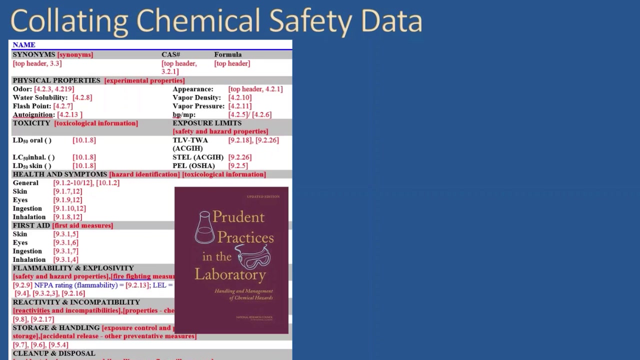 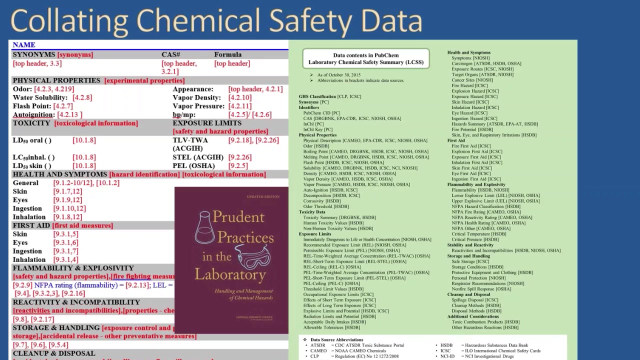 practices in the laboratory handling and management of chemical hazards publication. It was really a major step forward for laboratory chemical users and describe issues of scale related to laboratory use of chemicals. It provided a set of properties and a format to be used And the PubChem LCSS has more or less mirrored that content as a subset of information that. 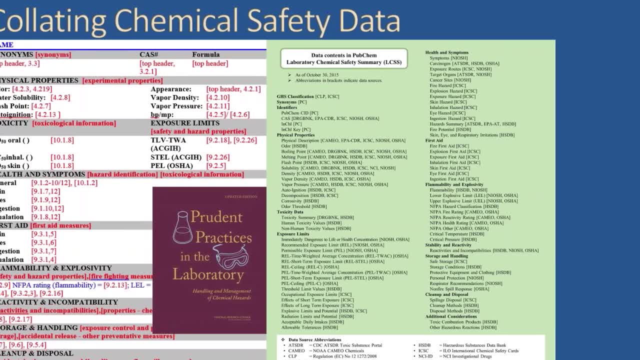 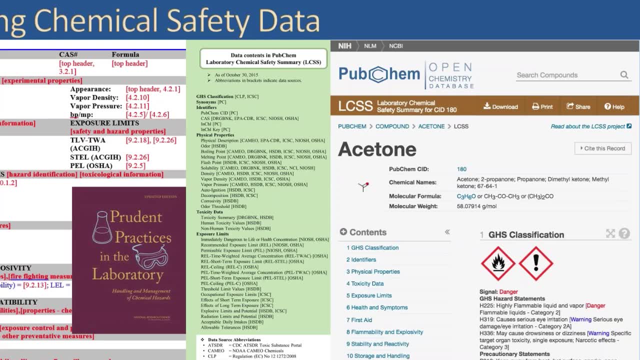 is available within PubChem as a whole. It includes various types of hazard and safety information, such as flammability, toxicity, exposure limits, exposure symptoms, first aid handling and cleanup. This evolution is important technically, but also culturally, because chemists have been 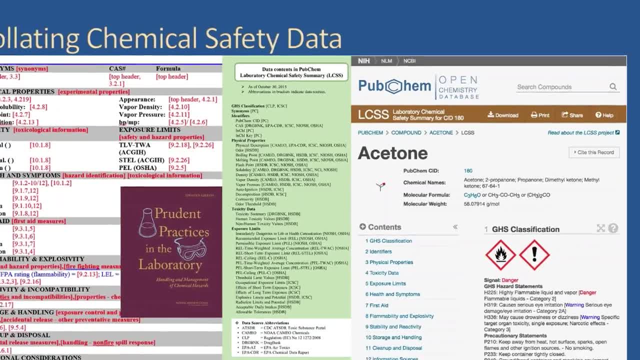 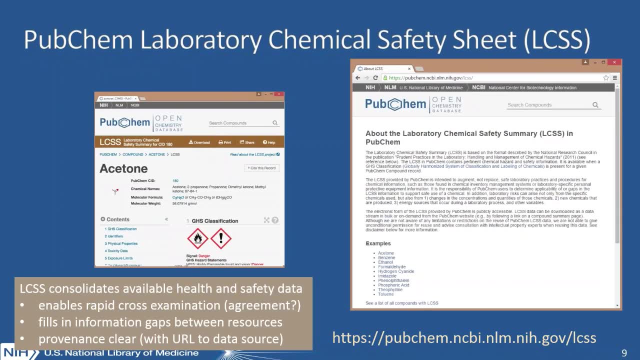 traditionally disappointed by the limited value of the MSDS. So what this you can imagine is the LCSS enables all the available health and safety information, or a useful subset of this, and making it available for ready use. One of the reasons why this is important relative to PubChem is that it provides a fair degree. 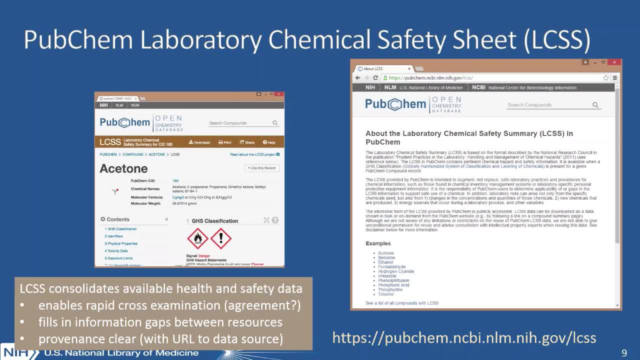 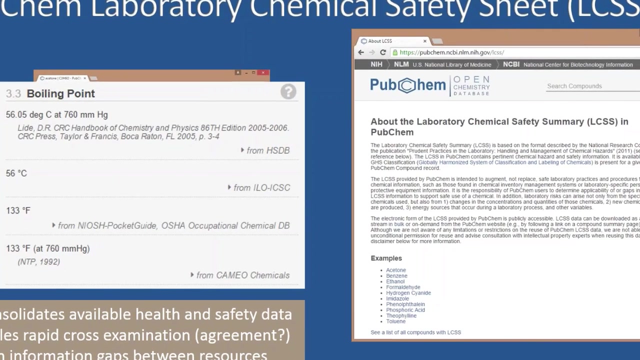 of breadth of information and really helps to move chemical safety information resources from the limitations of the 20th century paper media. So this is a very important aspect. So if you look at a typical property such as boiling point, you can then see who is providing. 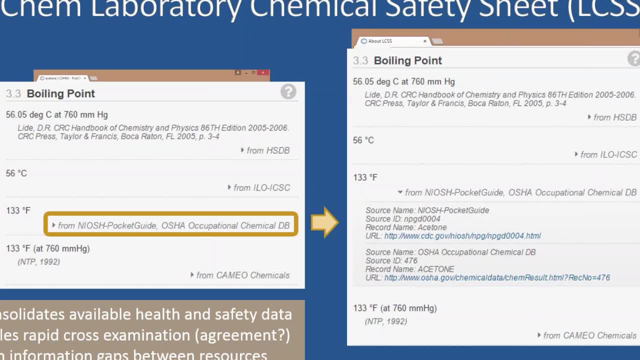 what information from various authorities. So if you look at a typical property such as boiling point, you can then see who is providing what information. So if you look at a typical property such as boiling point, you can then see who is providing what information. 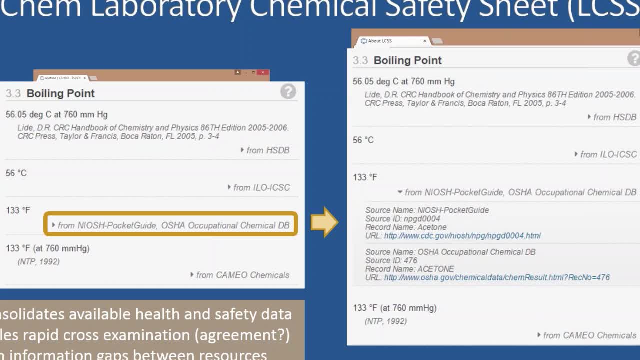 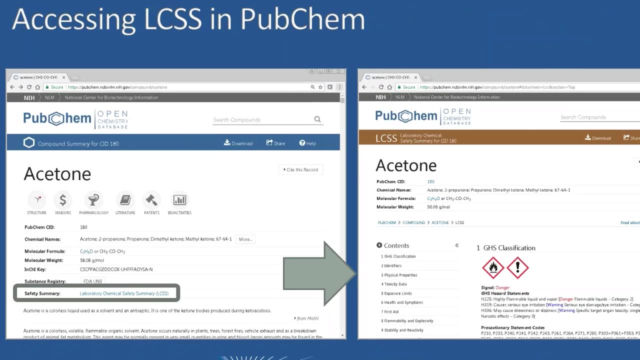 A common hazmat rule is that three sources have to agree on a property before an operational decision should be made based on that property. So with PubChem's collection of safety information allows for a direct comparison of authoritative data sources. You can access the LCSS in PubChem quite readily from any page that has this content. 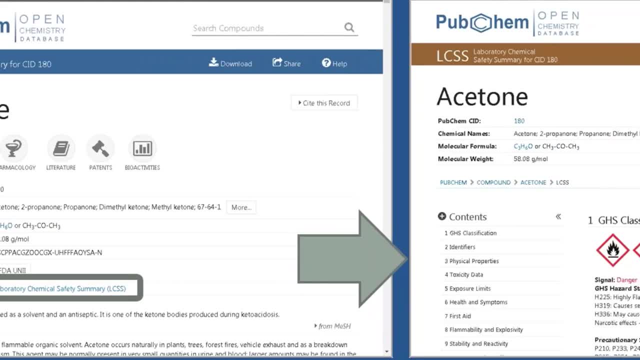 You'll see a safety summary link inside the page, Which will then give you a link to the public safety summary. You will then see it there. It is a very good way to provide info, useful information and tools for the public safety data sources. 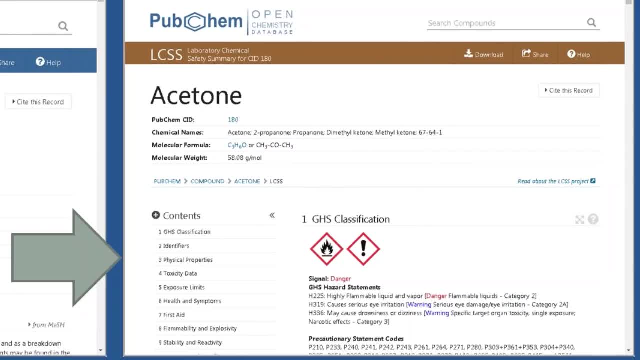 So PubChem offers this laboratory chemical safety summary data view for that same record, but the content is reformatted in such a way that is more in line with the GHS SDS sheet, but also to make for easy comparisons the information content. 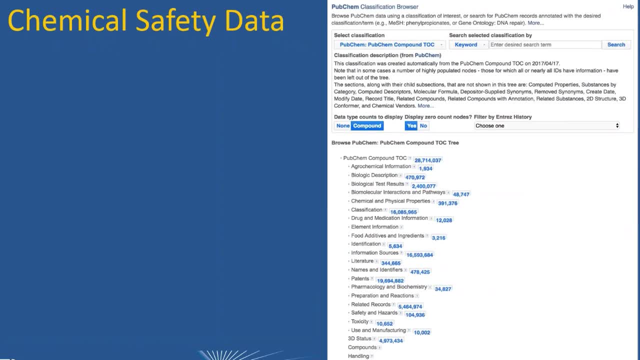 There's a fair bit of chemical safety data content inside PubChem. What you're looking at here is a data view from the PubChem classification browser where we're showing a classification tree for our PubChem compound table contents, Basically for the various information pieces inside PubChem. you can see that. 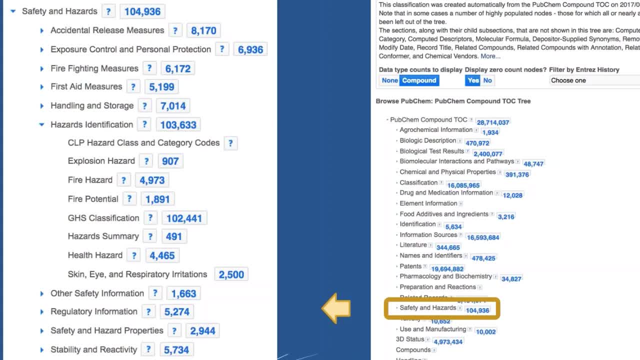 we have over 100,000 records with safety and hazard information content. The numbers you see here are the number of chemical compound records inside PubChem that contain certain types of property or property types that contain safety and hazard information, For instance for GHS classifications. 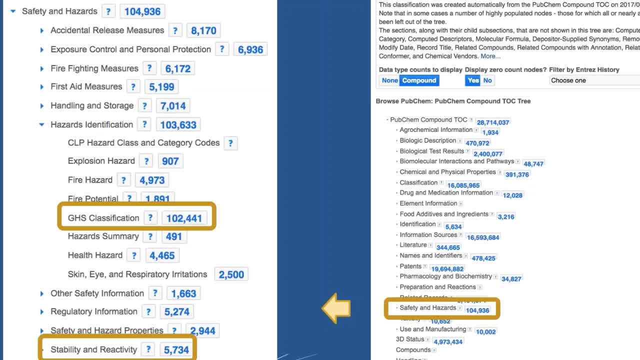 there are about 102,000 chemicals that have this type of information content. In addition, you can see that, or, in contrast, stability and reactivity information content is only limited to about 5,700 records, most of this coming through the National Library of Medicine's hazardous substance data bank. 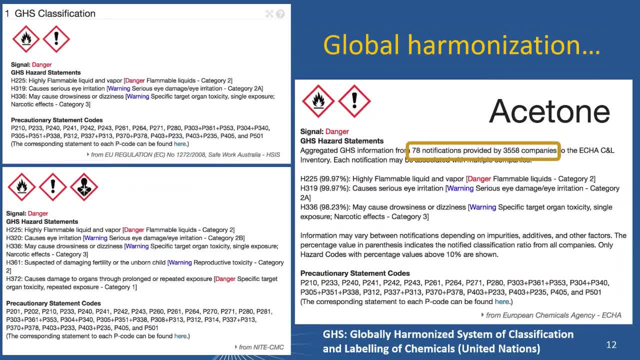 HSDB system. So in terms of global harmonization, you might find that the global harmonization is a little bit more complex than the national library of medicine. You might find that different data sources provide different degrees of GHS classification. Nice thing here is that PubChem has provided the subset of the 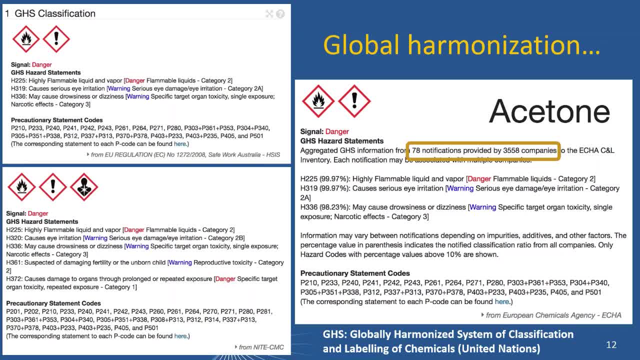 GHS information contents available. Perhaps important to this is the information content that comes from the European Chemicals Agency through the REACH efforts that they have there in Europe. One thing that you'll notice is that PubChem records will aggregate the content. so if you see here for acetone, there's 78 different notifications provided by. 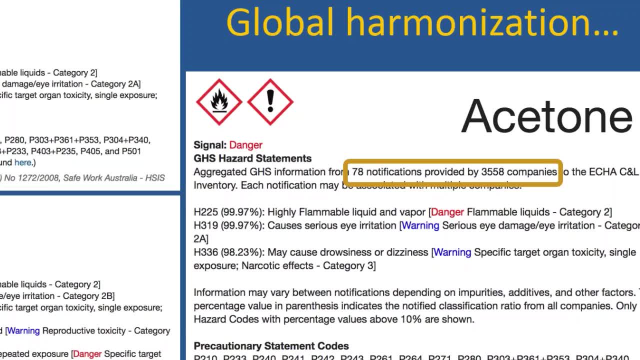 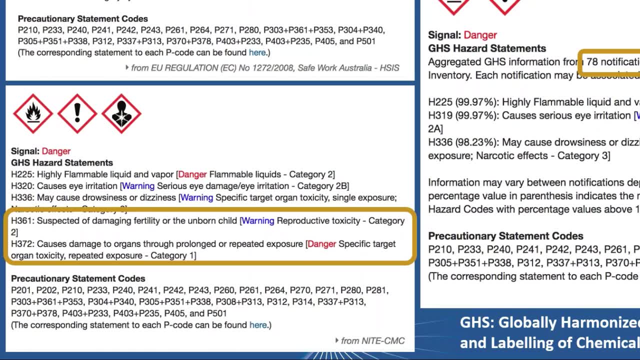 over 3,500 different companies. But you can see that when you compare this information content between the different sources, some data sources, such as that from the, the Japanese night data source, includes additional GHS hazard codes that you don't find for other records. So, in part by being able to 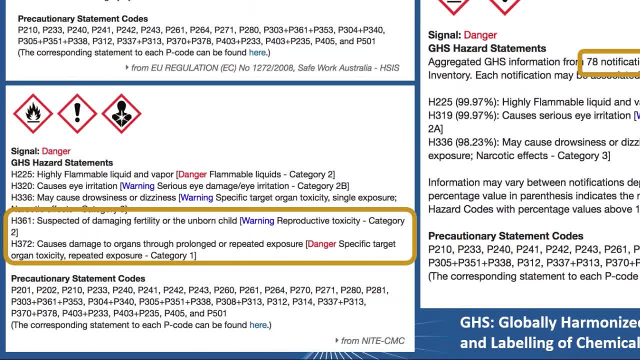 compare these different data sources, you can see that PubChem is able to do that And then, going back to the original data source to find out why, perhaps, that they have selected these different hazard codes, it can provide you more informed information in terms of decisions. 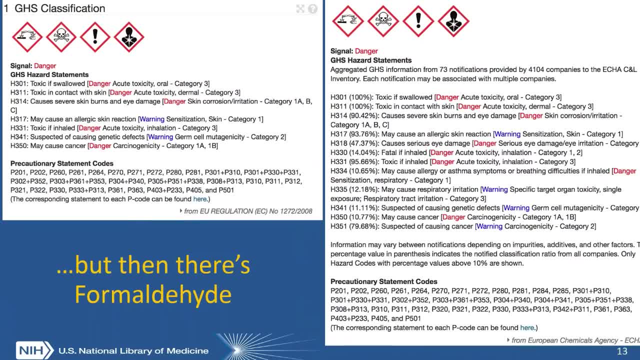 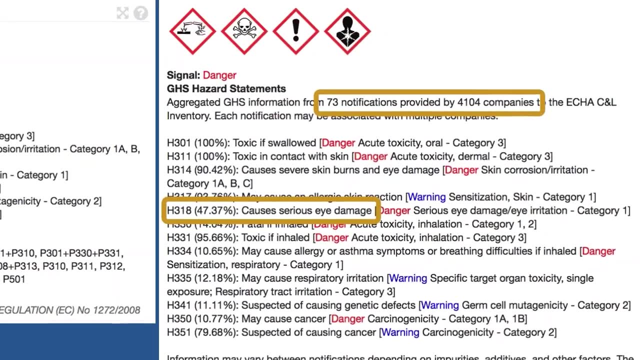 However, there are some issues with some of the information content that you can get through PubChem, in part because a chemical structure record could have multiple forms of an entity associated with it, As we see here. in the case of formaldehyde, there are over 4,000 companies providing different. 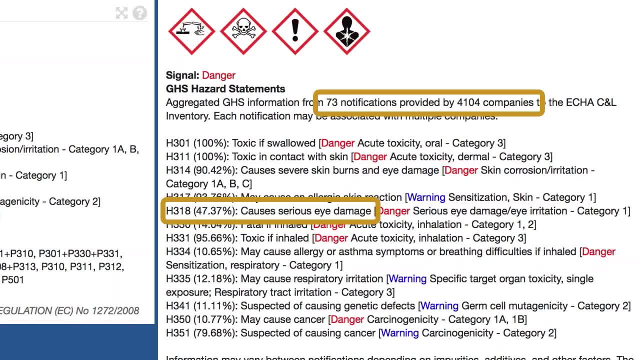 notifications and we had to provide a. we aggregated this information content and let you know what percentage of these notifications that are coming from. these companies are reporting various types of codes- hazard codes. They may correspond to different forms of the same entity. that is of importance to. 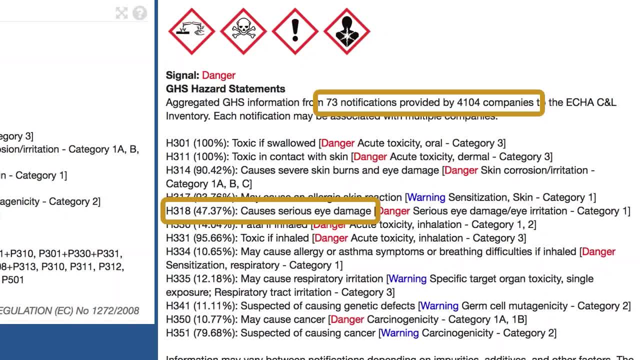 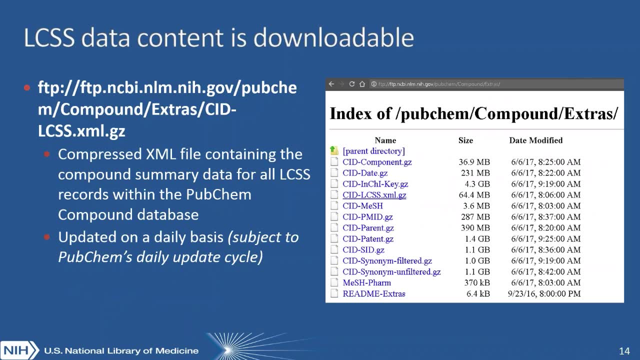 your use case or may not be important to your use case, So you'd have to examine and see what are the different records and types of information content that's available. A neat thing here is that PubChem opens up new opportunities for using safety data. 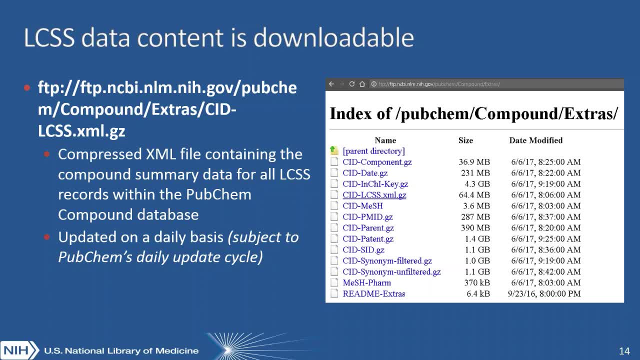 in a practical way by giving safety information in a very customized form via data streams. In fact, you can download the entire content. In this case, you can go to the PubChem FTP site and you can download a gzip compressed XML file that has the entire content of what. 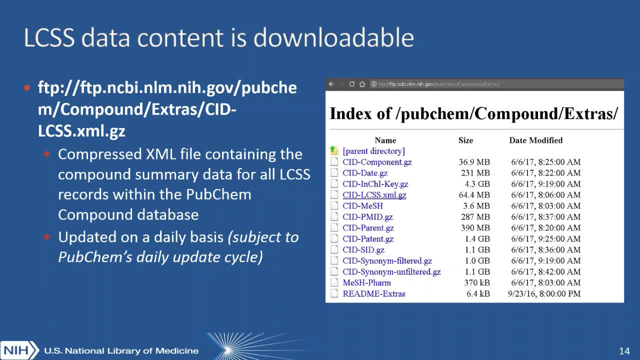 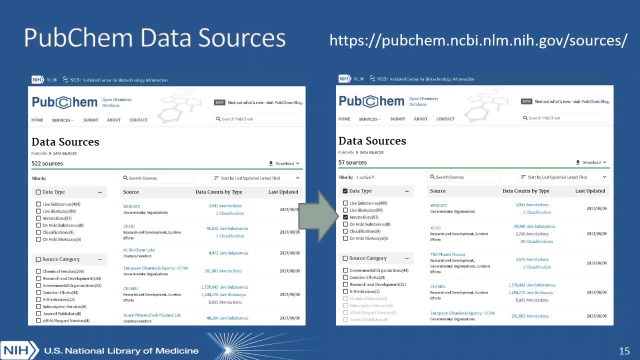 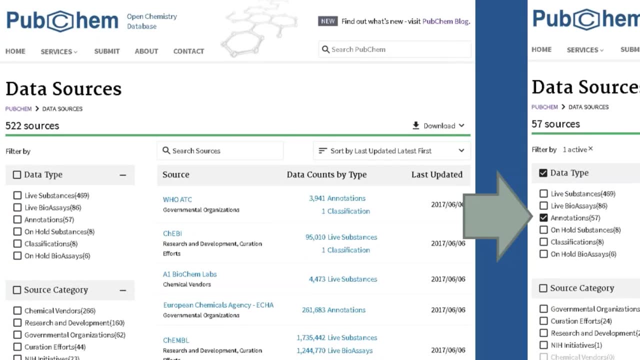 PubChem knows relative to LCSS And we update this on a daily basis. We also provide extensive provenance information where you can explore our different data sources and, for instance, limit them to annotation sources. So, out of the 522 data sources in PubChem today, 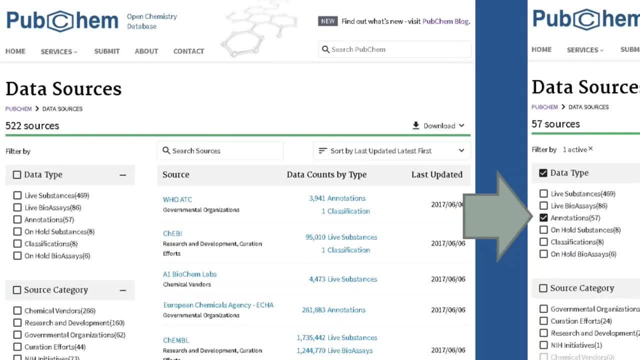 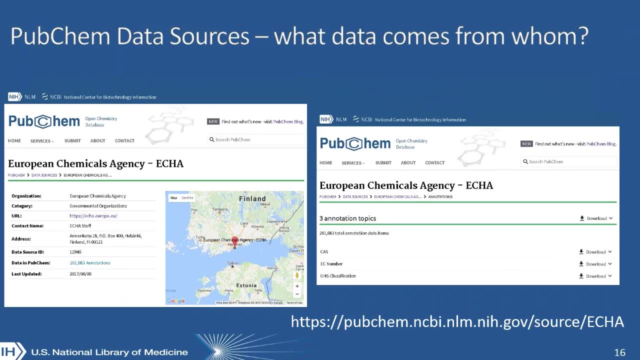 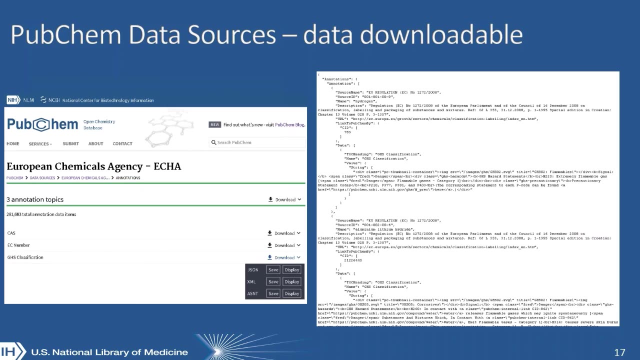 there's 57 that provide annotation content And you can examine each of these individual records. So, for instance, for the European Chemicals Agency, you can see that they provide us various types of information content, such as GHS classification information, And you can then download that content in a data stream. that may be helpful and 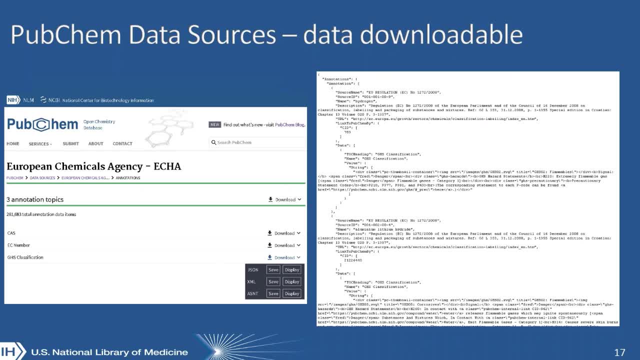 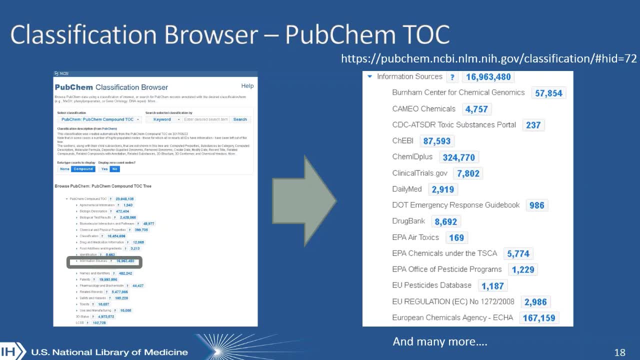 informative for your purposes. You can also download this information content on the fly. The earlier PubChem table of contents also lists the information sources so that you can see how many chemical records have information from particular data sources. So in summary, the PubChem Laboratory Chemical. 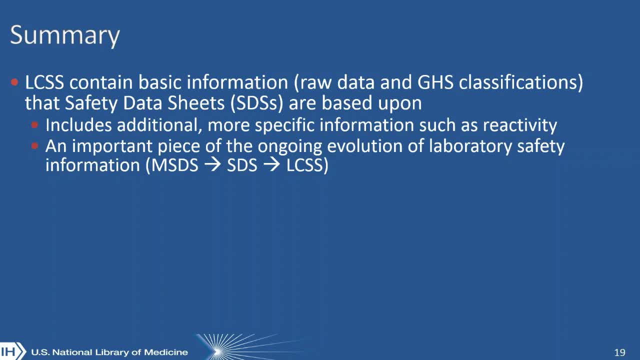 Safety Summary contains basic information, raw data, GHS classifications and more that are important for you to make informed choices or to locate information sources to make informed choices. It's also an important piece of the ongoing evolution of laboratory chemical safety information that helps you move away from paper and more. 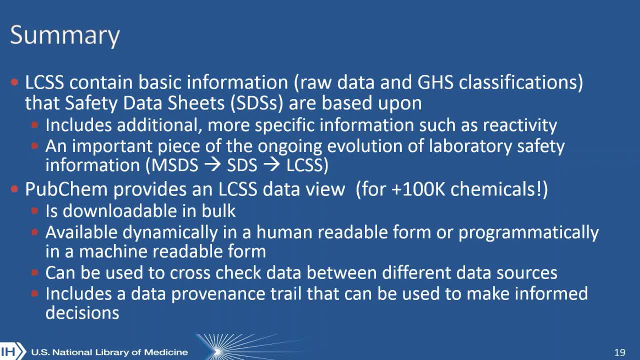 towards a simple way for you as a human to read that content, compare that content and to work with it in a computer readable way, In part because it's downloadable in bulk and we have quite a breadth of data: over 100,000 chemicals, but also a fair bit of 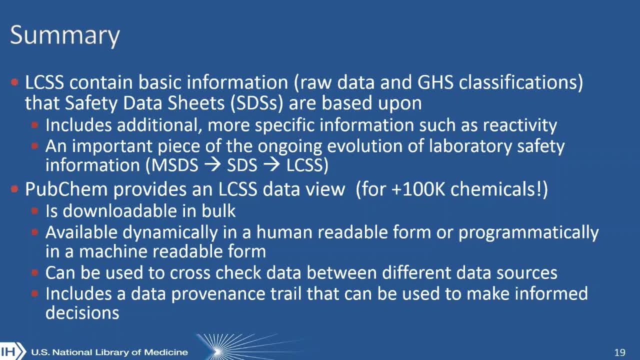 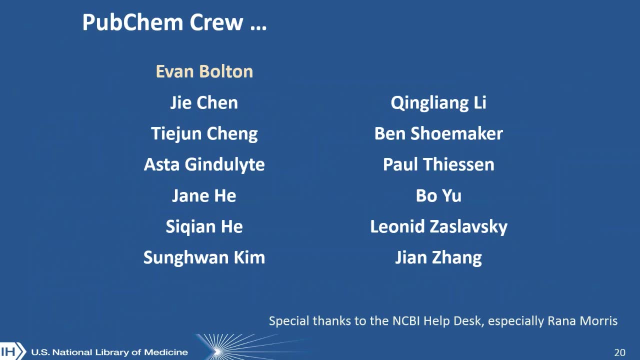 depth for a number of entities which have other properties and information content. that's important. It also provides an extensive provenance trail that allows you to understand which data sources that are authoritative and how we do the data linking. So the work that you saw here today wasn't just my work. it was from the various 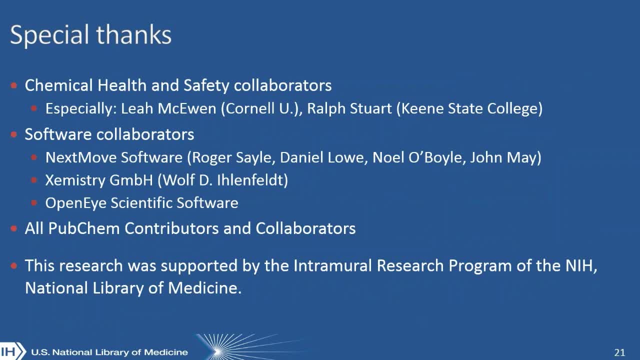 members of the PubChem group, but also in part due to our collaborators, especially a shout out to Liam McEwen and Ralph Stewart, but also our software collaborators, including Nextmove Software, Daniel Lowe and others, but also our PubChem data contributors and collaborators. This 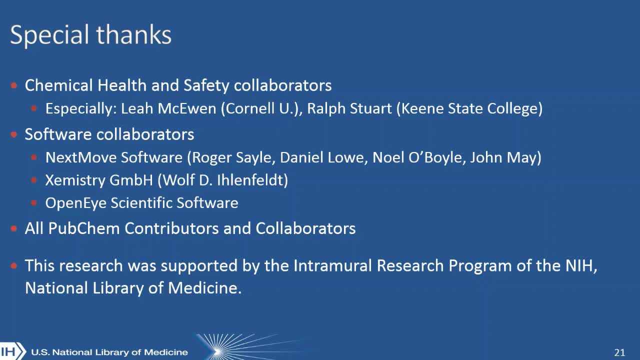 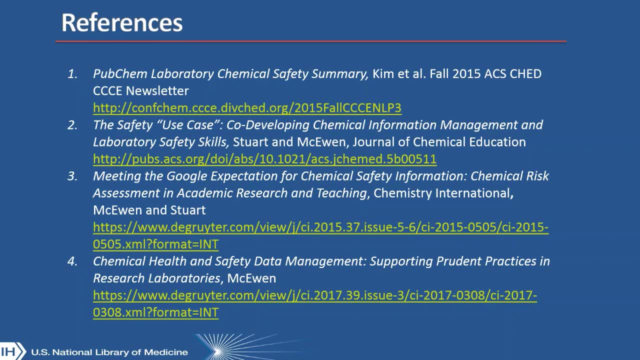 work was also supported in part by the Intramural Research Program here at NIH, And I've included several different references here for folks to get additional information about what was presented today, And I'd be happy to entertain any questions at this point in time. Thank, 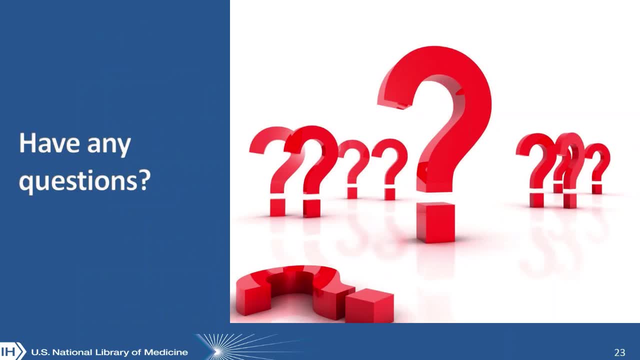 you. Thanks, Evan. We do have one question. in the questions pod It says you mentioned that the LCSS collection is updated daily. Is there a way to get more information about the collection? I'm not sure if you can answer that question. I'm going to go ahead and ask you a question. 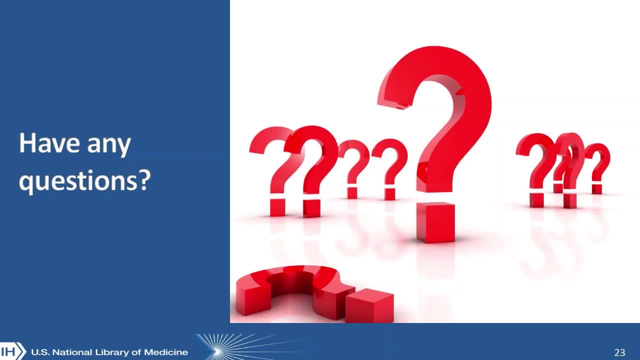 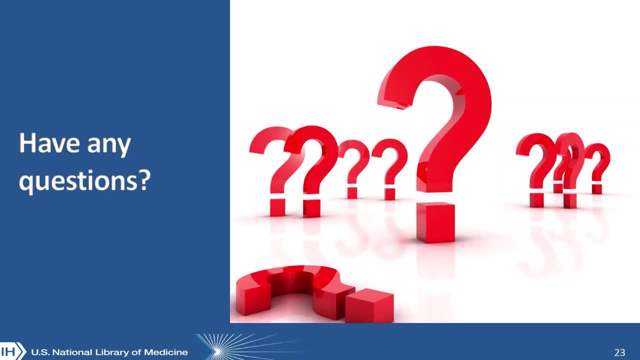 for a particular chemical. So in most cases the LCSS information is not changing on a daily basis. However, errors that people make in the LCSS could be updated at any time. It's having that update cycle, but also having inclusion of content on a regular basis allows us to keep up to date. 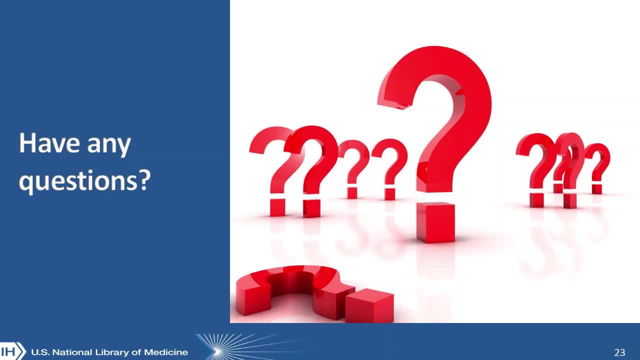 in which other changes that are made through the выход of new items. Uh well, here's just one. that is just a to-do list. within DB staan If somebody had throughout the information enterprise, But as new information content is made available, it then gets added and then one can access. 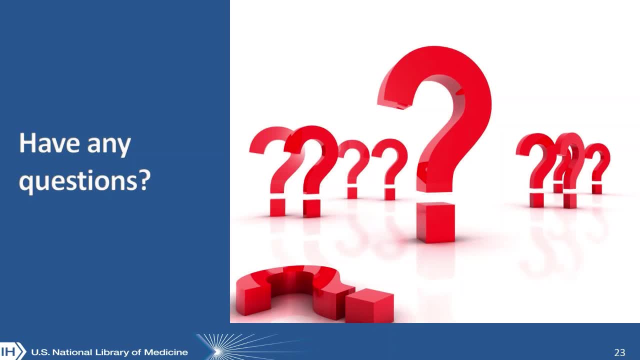 that additional information content. Okay, we have another question. In the aggregated data, for example, when there are 73 sources for the hazard codes, how do you delve into the 73 that were aggregated? In other words, how would you see the original reports? 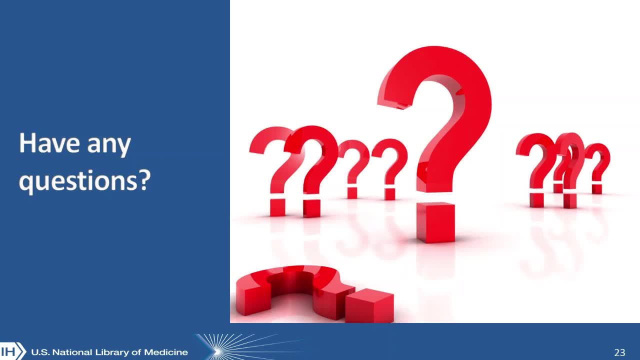 So this is to rephrase what I heard in terms of question: Can you access the original information content that was used to make up the LCSS inside PubChem? Yes, you can go back to the original authoritative information data source. all the URLs that: 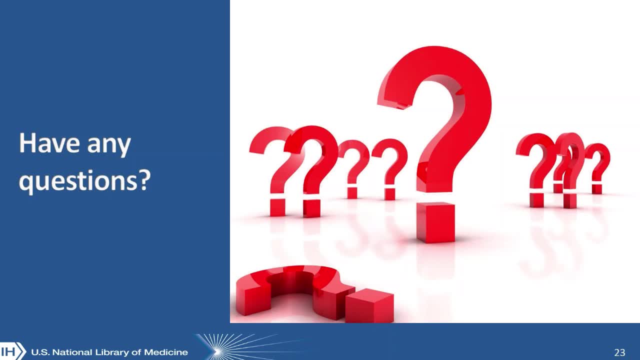 where the information content came from is available to you. In fact, when you start to see things that are different between different authoritative sources, you should immediately raise a red flag that you should go back and look at what they're talking about in terms of what aspect of that chemical or 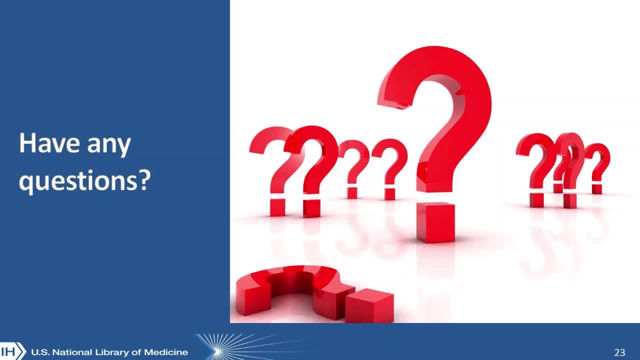 whether it could be a different phase of the material: gas versus solid, versus liquid, or a mixture form of that in some cases. Another question: If this is the evolution of the SDS, do you see LCSS becoming a standard for chemical reporting through suppliers? 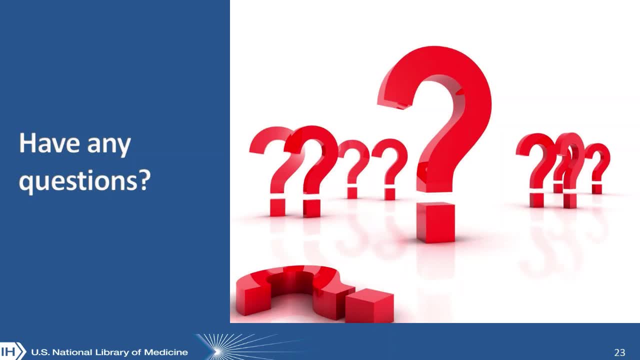 Well, I would say that suppliers oftentimes have a legal responsibility for the information content they provide, And while LCSS could be a standard for chemical reporting, it's not. It's not. It could become part of the information data streams that you see from suppliers. 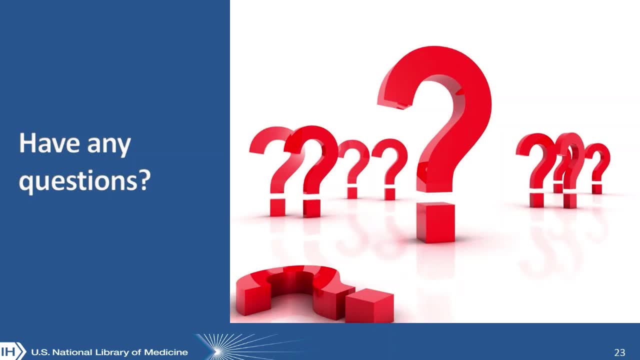 That legal requirement may provide some degree of separation as to what they want to report, and why Is there a version history tracking available? That is, can we know what information was available in December 2016 compared to today? No, not in the case of the annotations provided to PubChem. 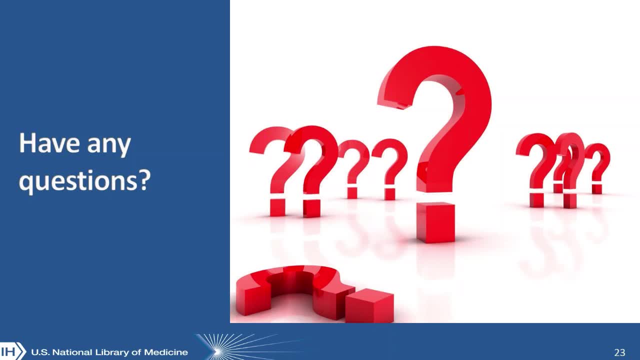 If it was in the archival part of PubChem, the answer would be yes. However, annotations such as these are not archived, So you would have to go back to the original data source to see what information they provided or to regularly download and compare the LCSS content that is found within PubChem. 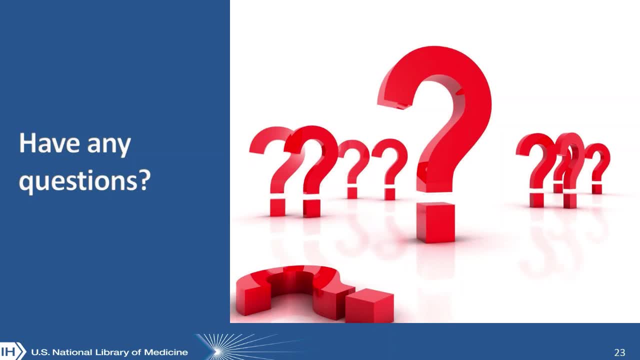 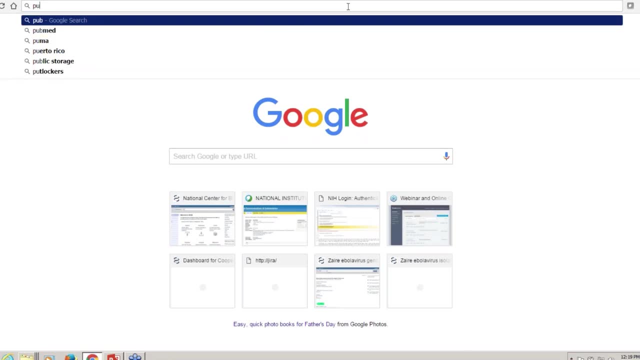 Okay, here's one that will put you on the spot, but I think it's a good idea. if you feel like doing it, Can you do a demo to show them how to get to this on the web page? Sure, So you can just type in PubChem. in this case, I'm going to Google and you can go directly. 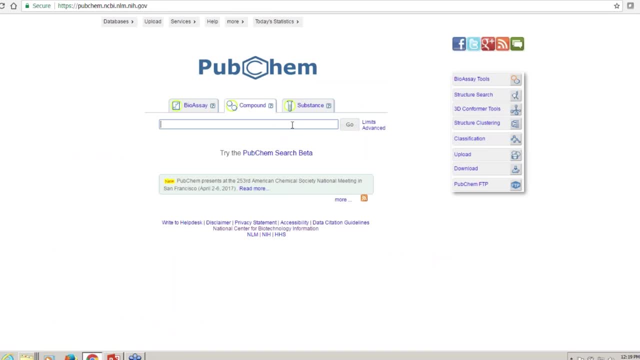 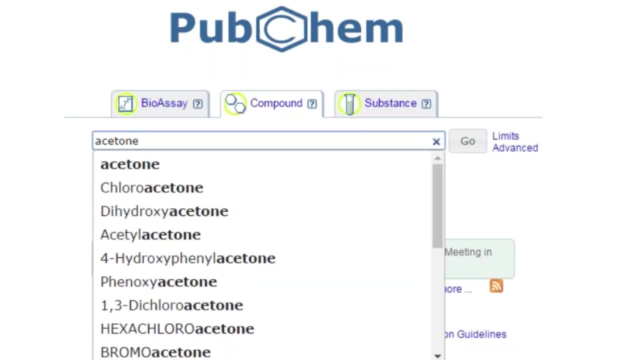 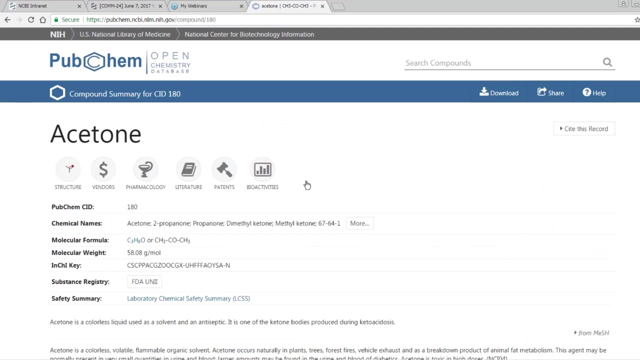 to PubChem. You can search for a record. oh, I don't know, would be a good one. acetone. it says a search within PubChem, you notice it finds a number of different data sources that are available. You can click on that record and you can see that the laboratory chemical safety summary. 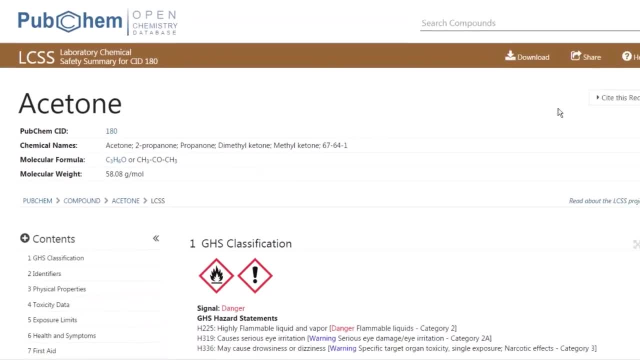 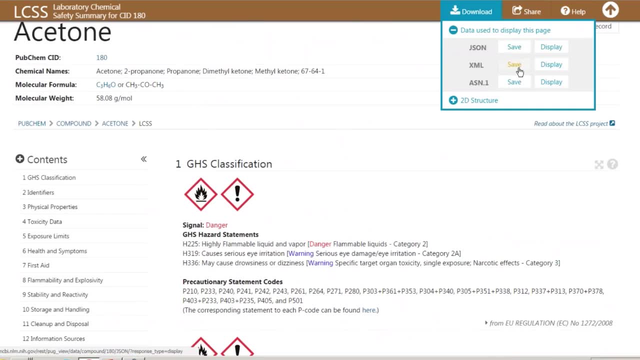 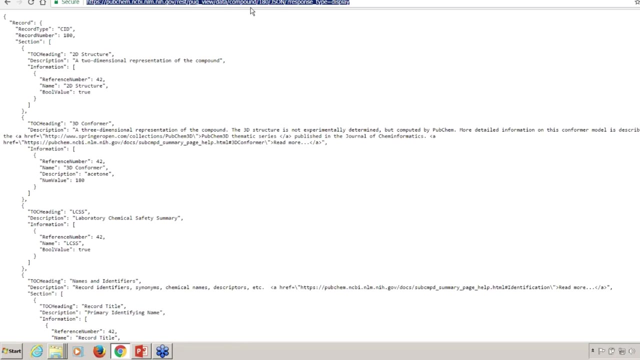 is right there. You can click on it and access what you see there. The neat thing is that you have a download button. You can always see the data used to display the page. you can download it in different formats and you can learn how to get these to pull them for a set of structures just. 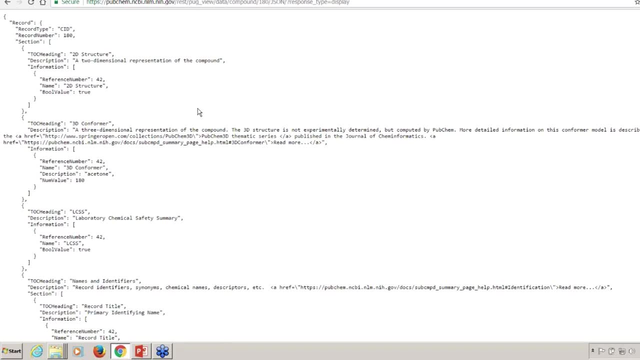 by looking at the URL that you see there. This information is in JSON format, which is not for humans to interpret but for computers, So if you had a programmatic access route that you were interested in, you have access to both of these. 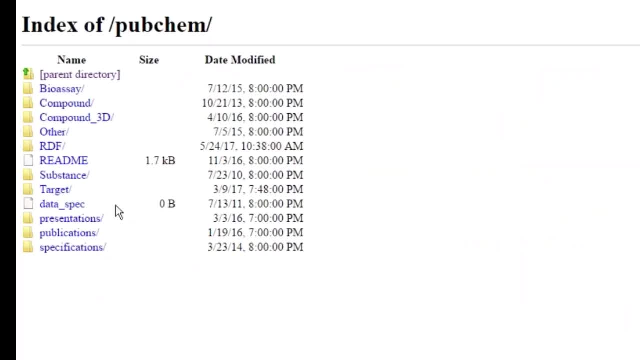 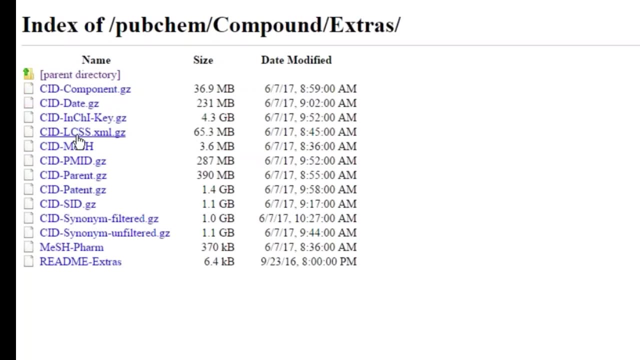 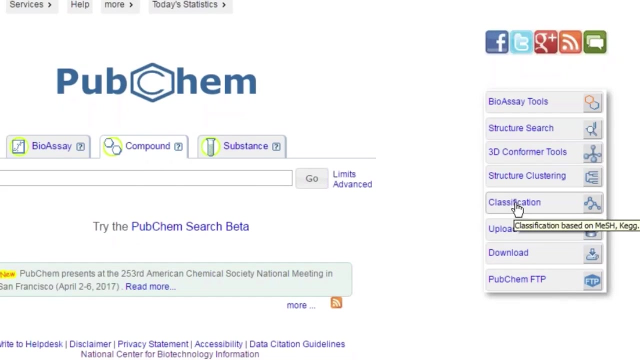 If you wanted to go to PubChem, you can go to the PubChem FTP site, You can go to the compound records in the extras folder and you can access the LCSS content directly right here. There's a classification tree inside PubChem. 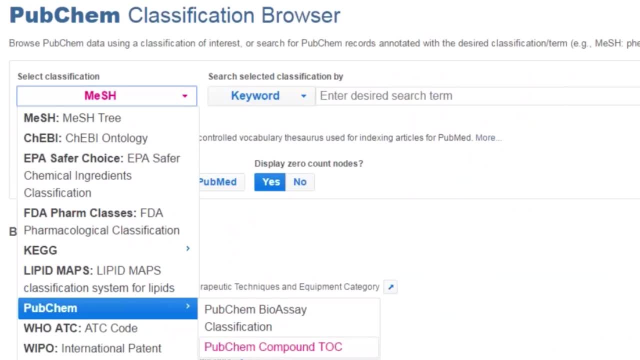 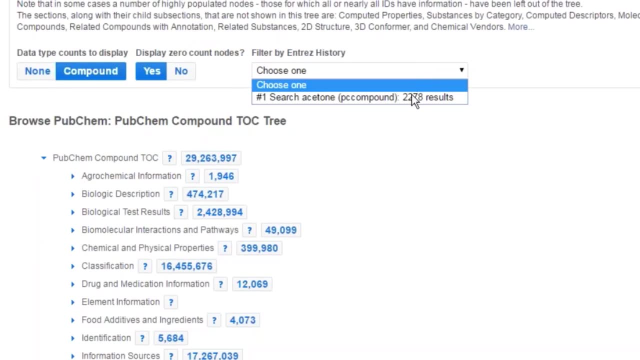 You can go down to the PubChem compound table of contents and you can see the various information that's available there. In fact, you can take a query that you had. In this case I did acetone just a moment ago. I can pull that record in and it'll do one on the fly and we see the various keyword. 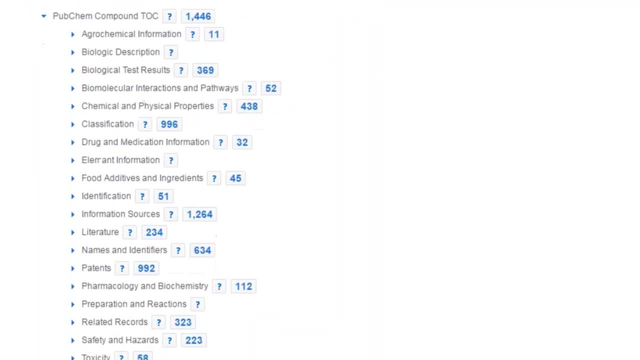 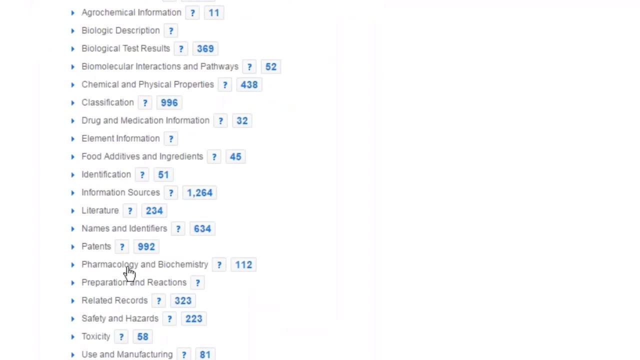 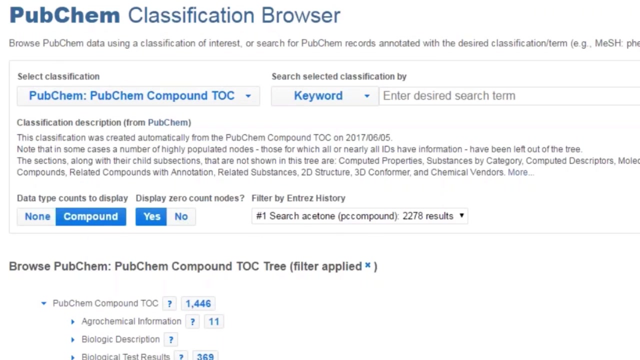 searches of acetone. There were over 2,200 records, but over 1,400 of these have some type of annotation content. Of these we can see that there is safety and hazard information for 223.. Oops, moving around some of the elements of my screen here. 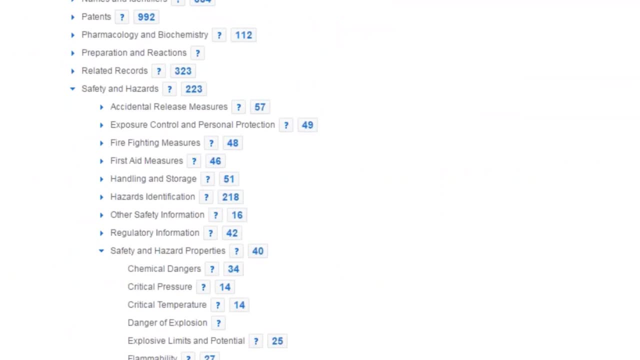 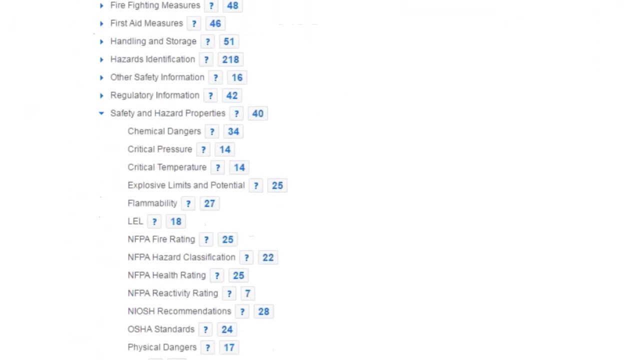 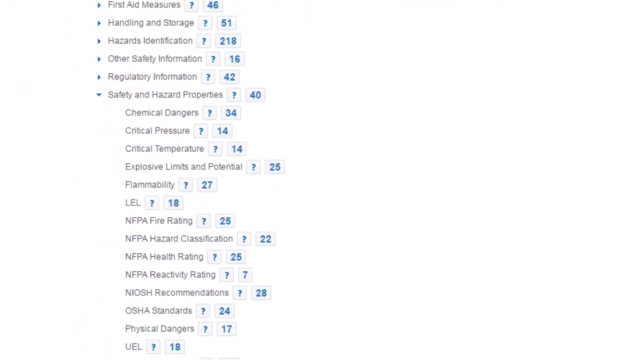 We can figure out how many have GHS content and I'm going to just do a turn off records that don't have any information. We can see various types of information that is helpful and useful for our purposes. We see 216 have an LCSS data page. 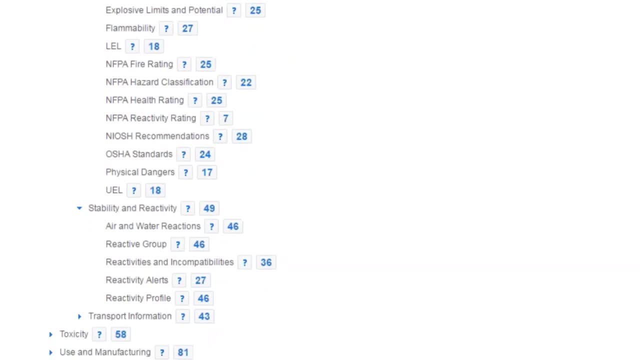 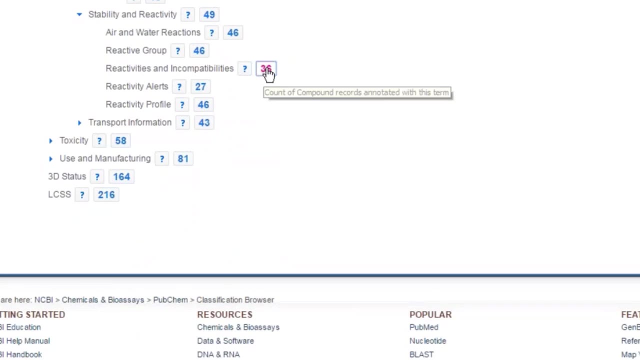 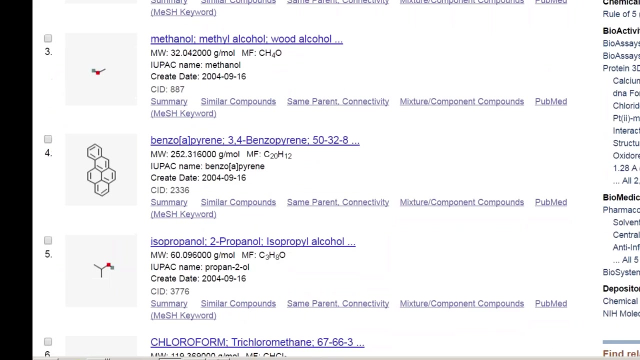 We can look for stability and reactivity content. So if we're interested in those that have reactivity content, we can look for stability and reactivity content. If we have reactivity and incompatibilities, you can click on that. In this case, we can see which records have it. 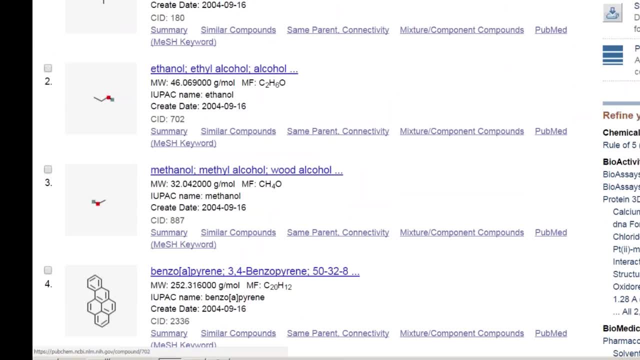 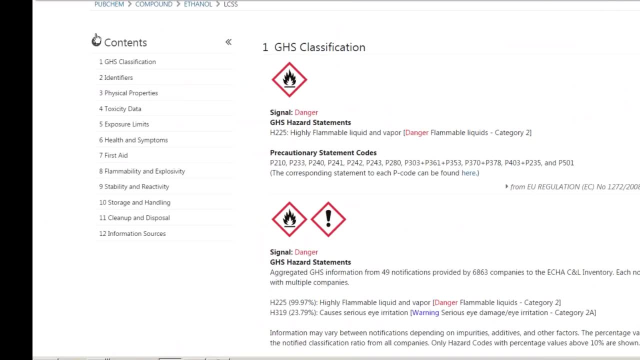 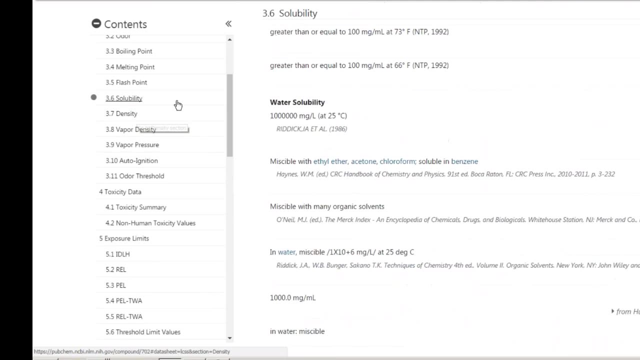 We have ethanol, methanol, various other types of records. A neat thing that may be worth exploring is that you can expand the table of contents and you can find other types of information that you may be interested in. Say you wanted to know about solubilities.